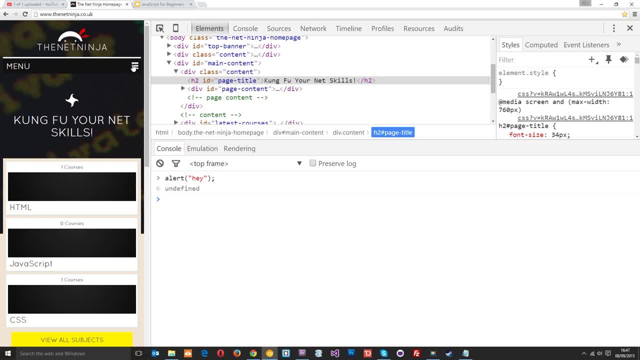 Essentially, I wrote a piece of code or a function that will do something when a particular event happens. Now, how do we write these events? Well, you can write them directly into your head. For example, I could say something like in here: add an attribute. 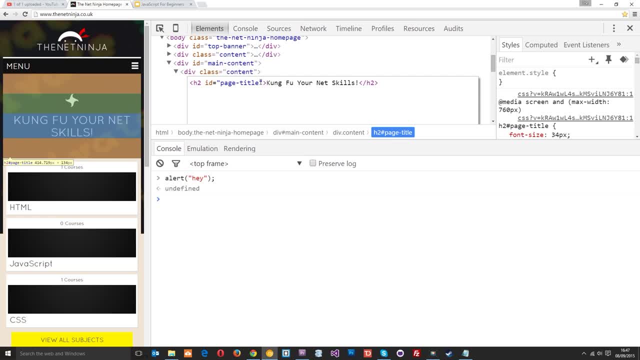 Let's just edit this HTML. I could add an attribute here and say: on click, that's the event name, equals alert. you clicked me, Alright, And we could do something like that. Let's just get out of here and try it out. 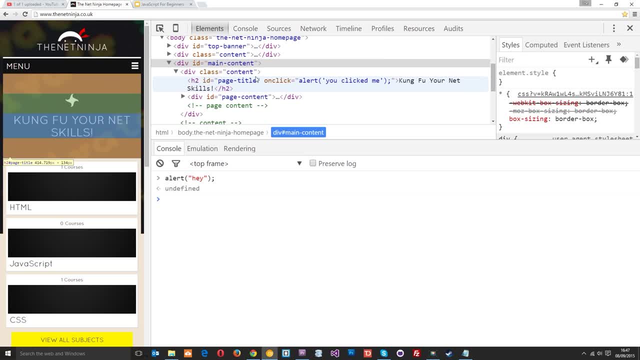 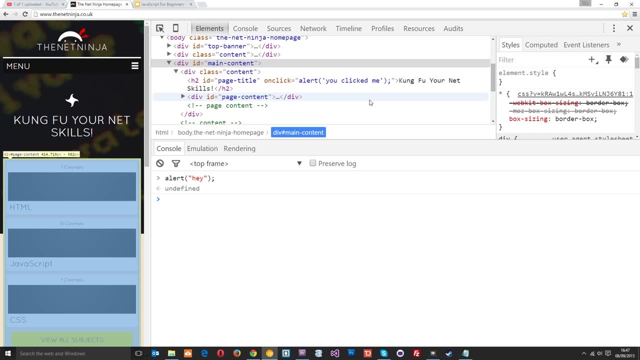 Now we get the alert. you clicked me So we can add events to elements That way. However, I don't like doing that. I think it's messy. It closes up your HTML. I think HTML and Javascript should ideally be kept separate where possible. 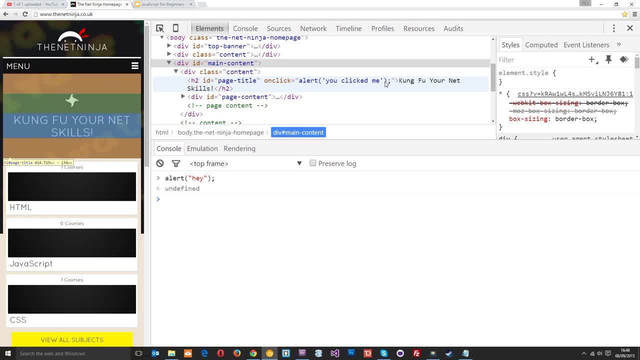 And imagine if you had some kind of bigger function that you wanted to happen when this was clicked. You're not going to want to write loads of Javascript in your HTML. And again, if you had the same event happening on multiple pages. much like this I have. 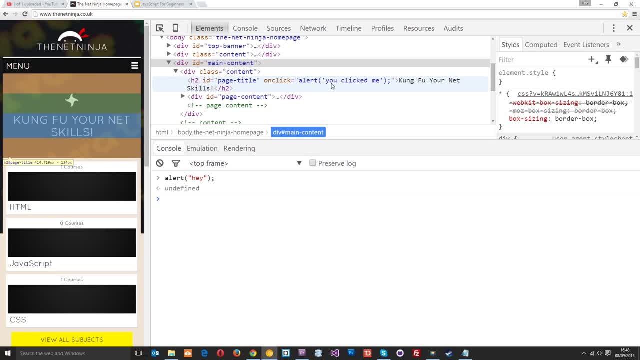 this on every page. I wouldn't want to write it on every HTML page. I'd just write it once in my Javascript code and then load that code into every page. Alright, So it's much easier to write these events or to react to these events in a Javascript. 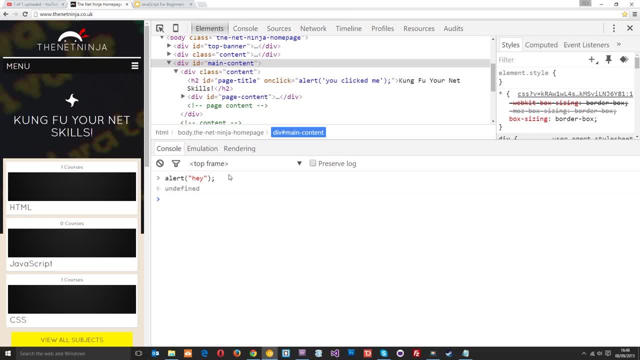 file, Alright. So how would we do that? Well, each element that we get in the DOM has these event properties, And there's loads of event properties. I'm not going to have time to go through all of them, I'm just going to go through a few here. 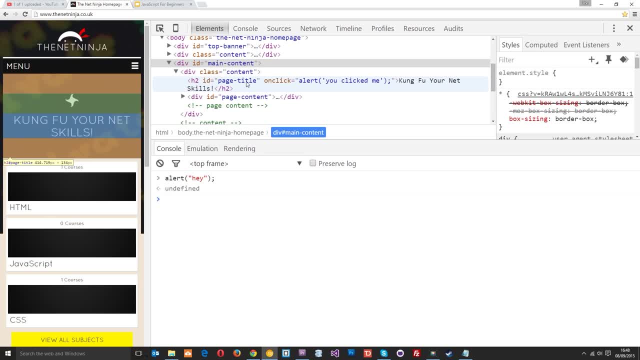 Right. But essentially how we do it is grab an element out of this HTML code, Right, And we're going to create an event to happen to. So, for example, let's just get rid of this, Let's edit the HTML. 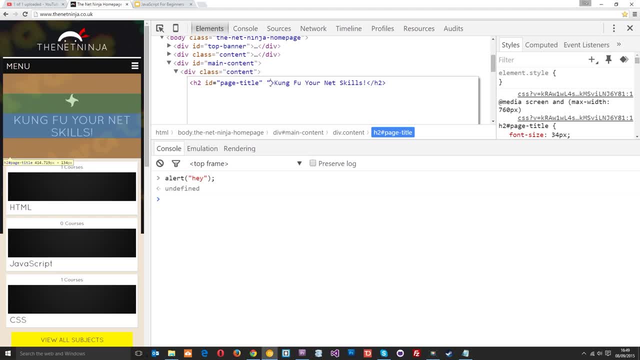 We'll get rid of the event there. And let's say, we want to add some events to this H2 right here. Okay, The first thing we need to do is get that H2 element and store it in a variable. Alright, We know how to do that. 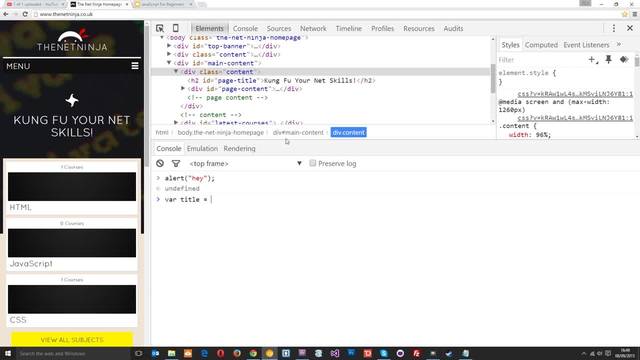 We'll create a variable var and we'll call it title, because documentgetElementsById- oops, wrong one, documentgetElementsById- and then the ID is page title, And now we've stored that in a variable called title. Right. 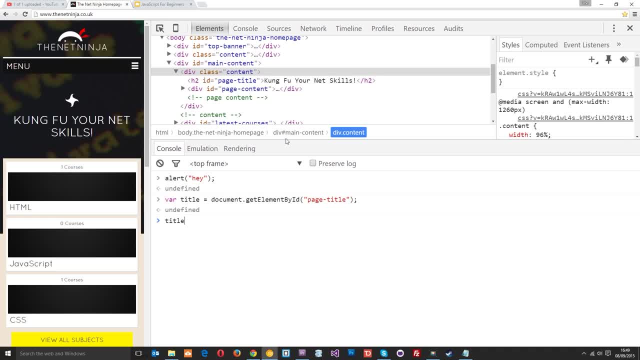 Now this title now has access to all these event properties And, like I said, there's tons. We can have: click events, mouse over events, load events- literally far too many to do a course on Right. What I am going to do is leave a link down below to a web page where you can see all. 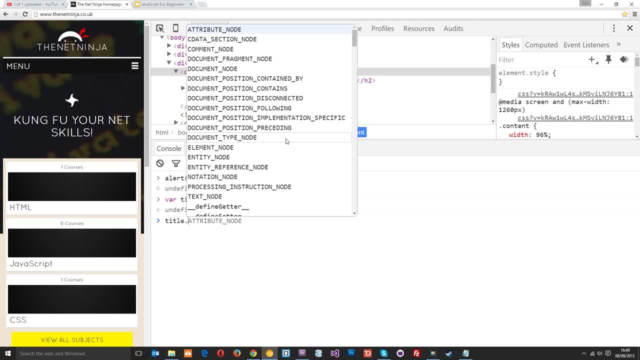 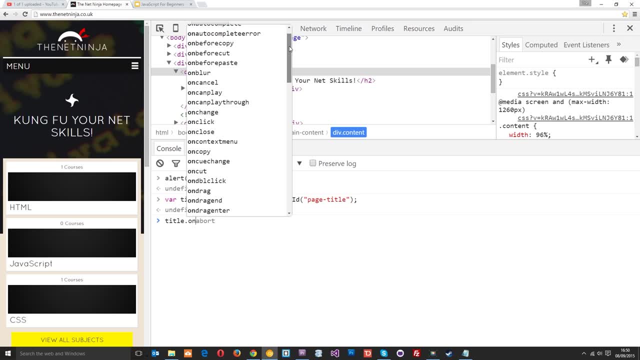 those events, But for now I'll just go over a few And I'll say the onClick event. In fact, if you write on and you're in Google Chrome developer tools, like me, you'll see a list of loads of different events that we can have here. 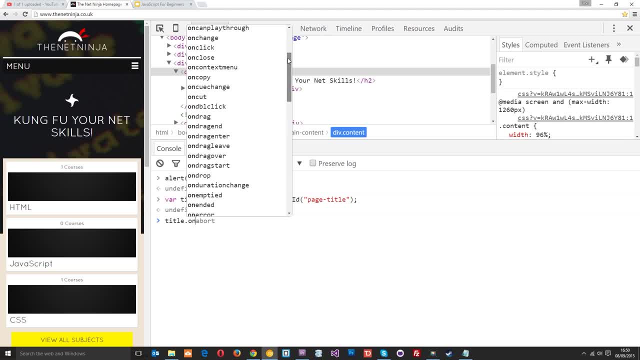 Alright, They're all on something generally. So what we'll do is an onClick event, And that's saying, when someone clicks this title element, I want something to happen, Right? So how do we write what happens? Well, we assign this a function. 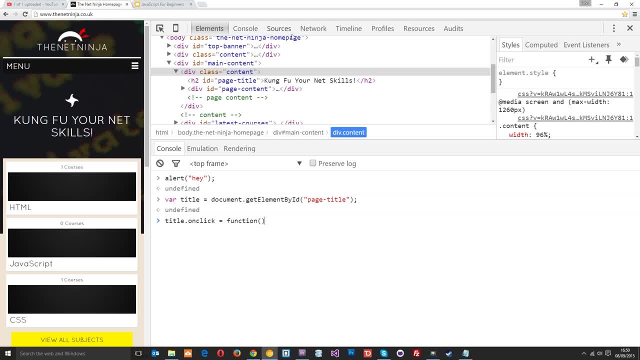 So we say it's equal to a function Like that, And this here is what's known as an anonymous function, because it's not got a name. Normally, we'd give a function a name, wouldn't we? You've seen that when we've discussed functions in the past. 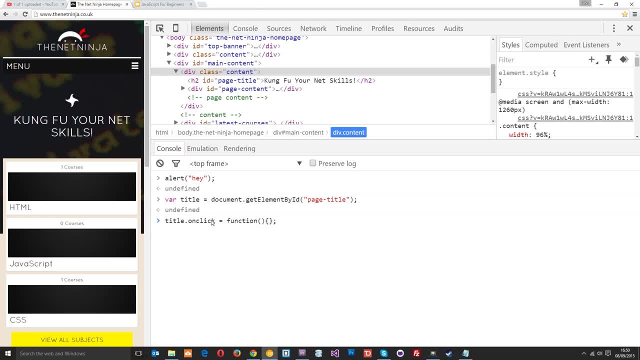 But in this case we don't need a name because we're just assigning this function to this onClick event And you might notice that we've got this semicolon at the end. That's because this is a statement, right here. When we normally declare a function, we don't have this statement. 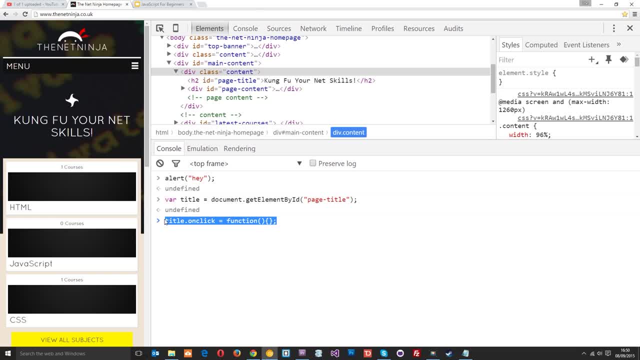 We don't have a function, We don't have this semicolon, But because this is a big statement with the assignment operator, we have to put this at the end. Alright then. So let's write this function. So I'll say that when this is clicked on, I want to alert you. clicked me. 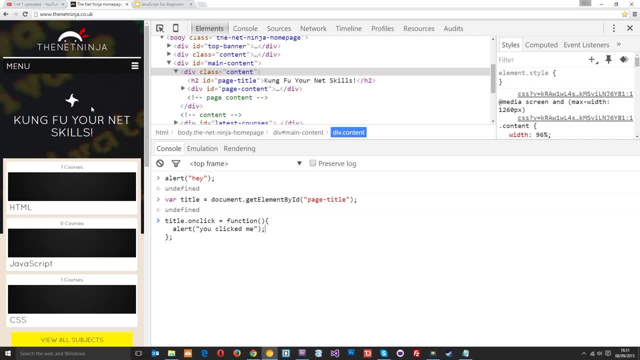 And you can have whatever code you want in here. Right, You could have code that swirls this around, zooms it off the page, makes it fade out. You can do whatever you want to do with this element. I'm just keeping it simple. 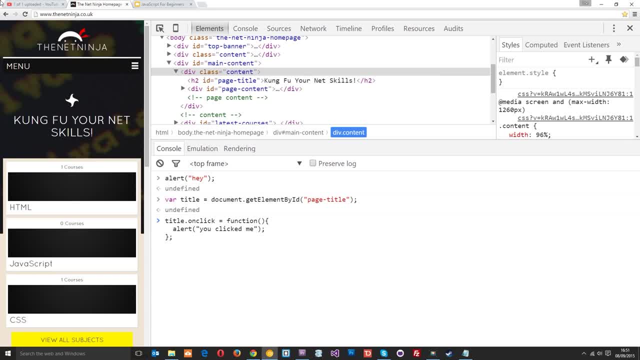 Alright. so now we've added that event dead simple Click enter And that function has been attached to this event. So when I click on this now we're going to get this alert, I'll press. okay, I can click again. 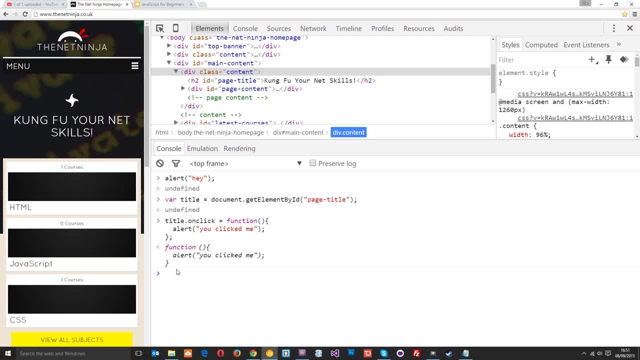 Get that alert. Okay, Cool, We've attached that onClick event to this element right here, And we can attach other events too. Let's do a titleonMouseOver. Okay, I'll click on that. There we go. That's another event, and this is an event which recognises when you place your mouse. 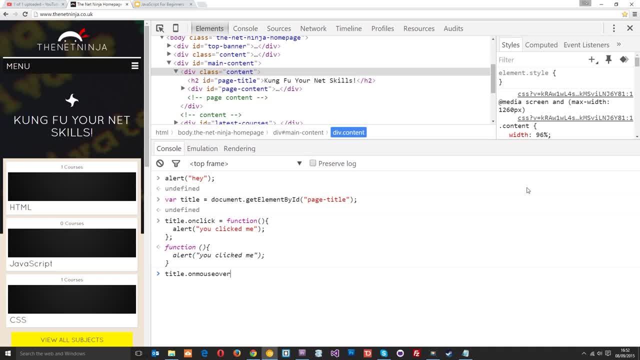 over the element. So I'll say: this equals a function and an alert will pop up again and I'll say: you hovered your mouse over me, winky face, dirty talk there. So let's save this and let's try it. there we go. you hovered your mouse over me, ok. 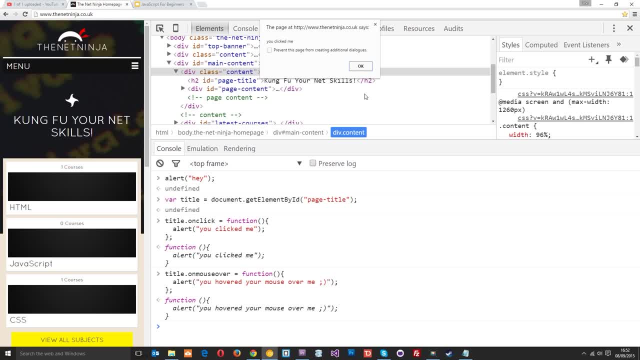 you hovered your mouse over me. ok, click, one's still there. you clicked me. awesome, Alright then. so they are JavaScript events. There is another way to do this, and that involves event listeners, And it's a method called addEventListener. oops, I thought I was typing that addEventListener. 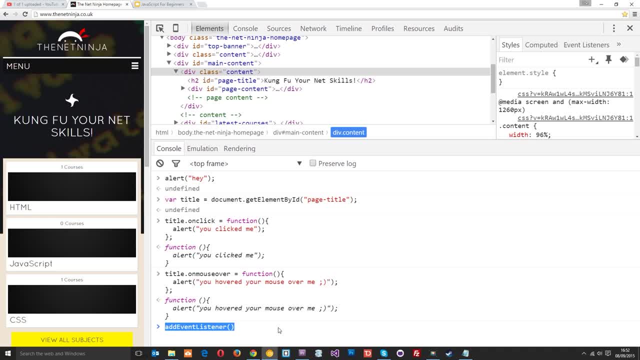 just like that, And this takes a few different parameters. but for the sake of this course and playlist, I'm not going to go into this, because they still have a few browser inconsistencies, particularly when we're dealing with Internet Explorer 8 and below. Alright, so maybe in the future, when I do advanced JavaScript courses, I'll include that. 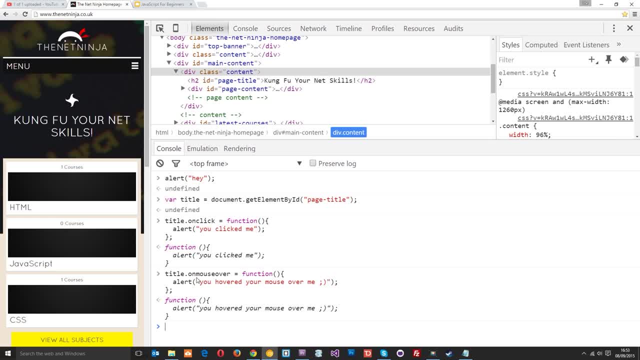 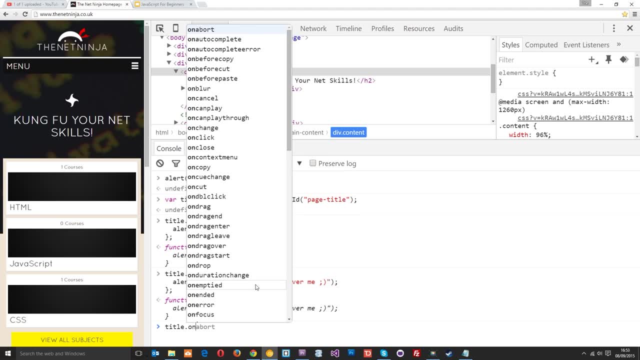 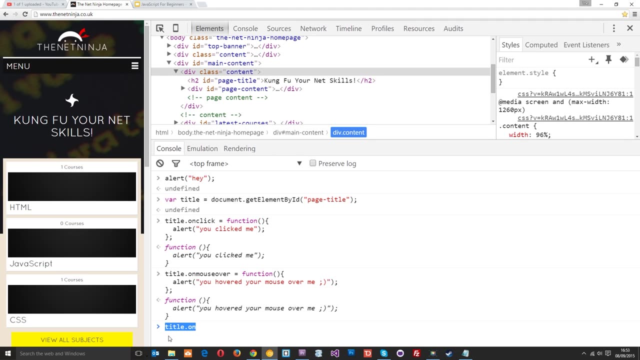 in there, But for now I think you'll be fine with it. So I'm going to end this video here and I'll see you in the next one. bye for now. Bye.